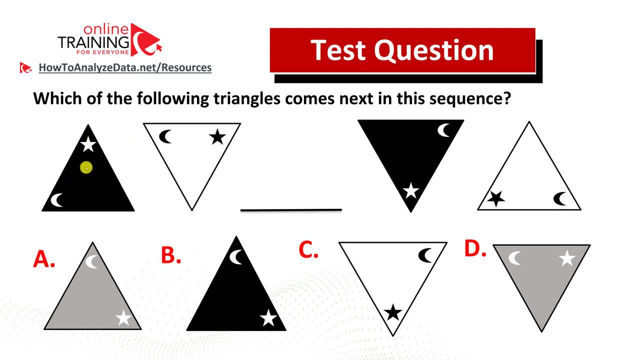 You also have a pattern of moon and star and moon and star. they move inside the triangle. So you see moon and star in the leftmost triangle, then you see moon and star on the top, then you see moon on the top and star at the bottom, and then you see both of them. 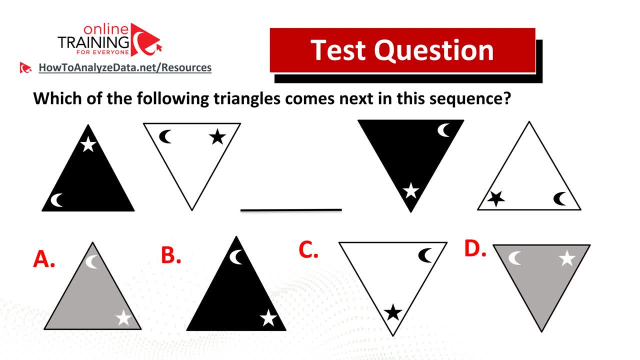 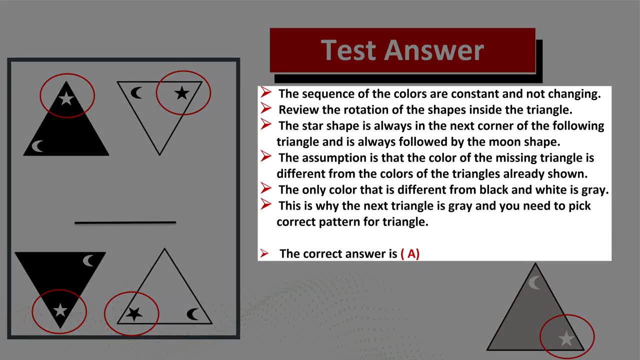 moon and the star at the bottom of the triangle. So now let's jump to the solution. We have already looked at the pattern of the colors and the sequence of colors is constant and is not changing, and we also reviewed the rotation of the shapes inside the triangle. 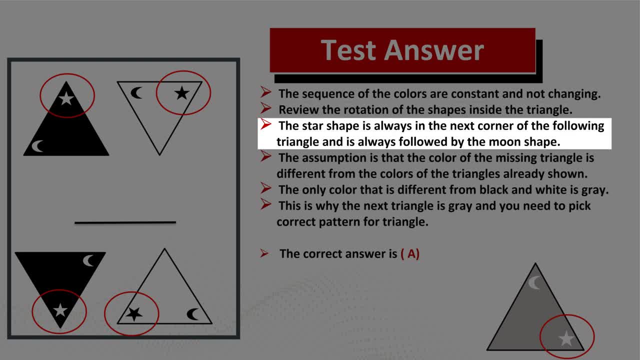 The star shape is always in the next corner of the following triangle and is always followed by the moon shape. The assumption here that the color of the missing triangle is different from the colors of triangles already shown and the only color that is different from black and 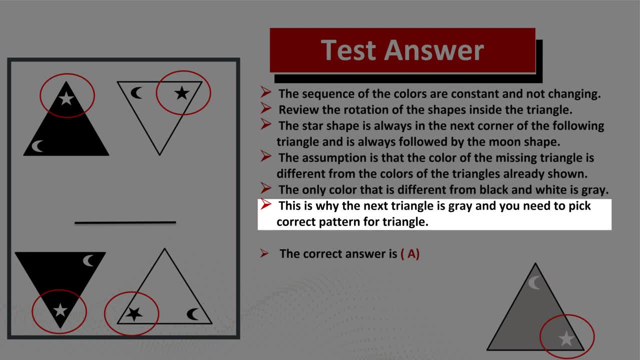 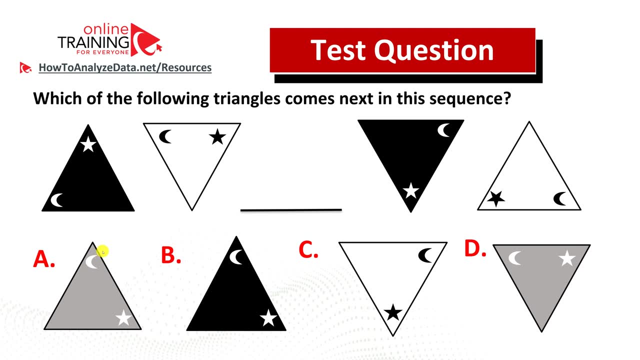 white is gray. this is why the next triangle is gray, and you would need to pick correct pattern for the triangle. so the correct choice here is choice A. there are two gray triangles here, choice A and choice D, but there is also a third pattern pattern that I did not mention because it will make things very obvious. 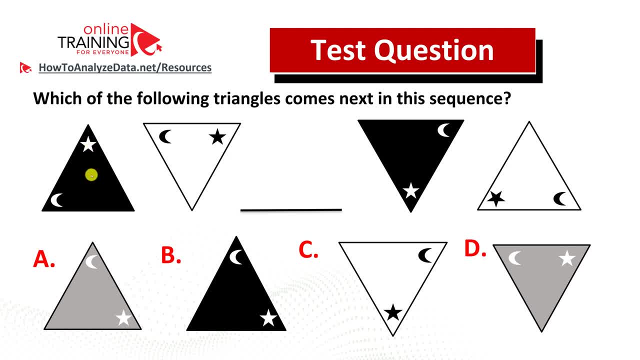 and this is the pattern of pointing. you see that the first triangle is pointing upward, the second triangle points down, so the next triangle in the pattern will be pointing up as well, and the only gray triangle that points up is choice A. hopefully you've nailed this question and now know how to see the patterns and 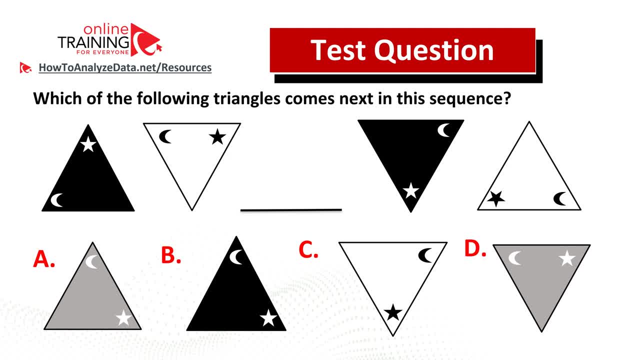 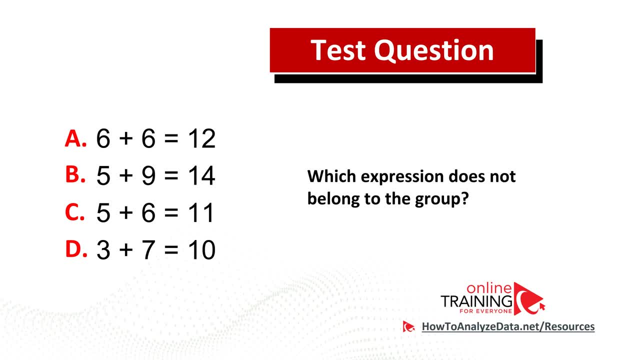 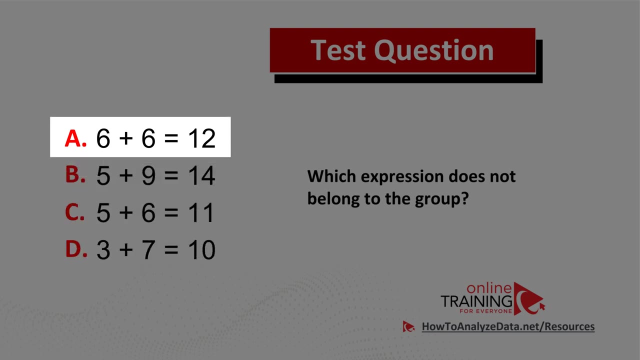 solve these types of challenges on the test. let's see if we can solve this challenge together. here is the very interesting and at the same time tricky question. you might frequently see on the test which expression does not belong to the group and you have four different choices. choice a: 6 plus 6 equals 12. choice B: 5. 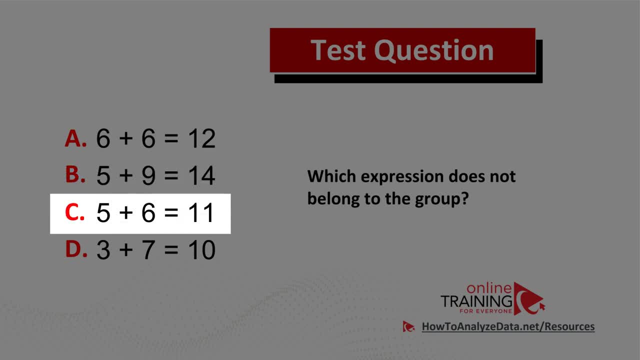 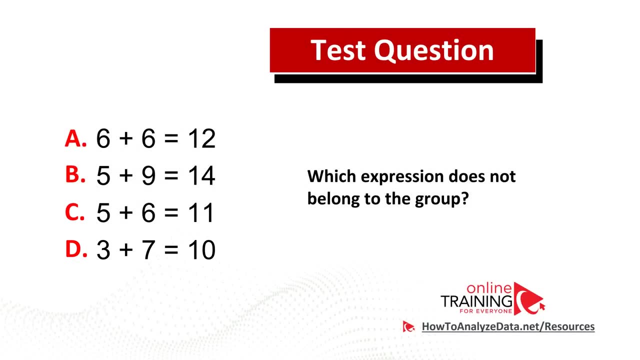 plus 9 equals 14, choice C: 5 plus 6 equals 11 and choice D: 3 plus 7 equals 10. do you think you know the answer? now might be the right time to pause this video to see if you can come up with the answer on your own. give yourself a. 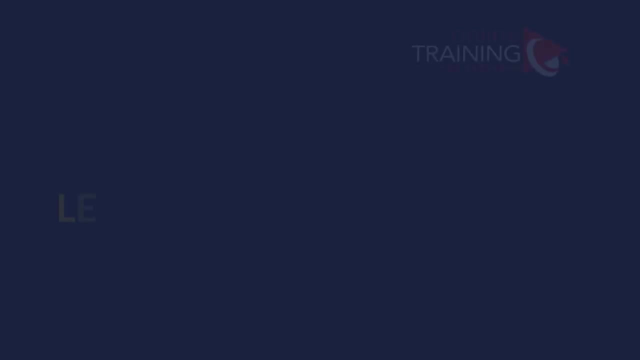 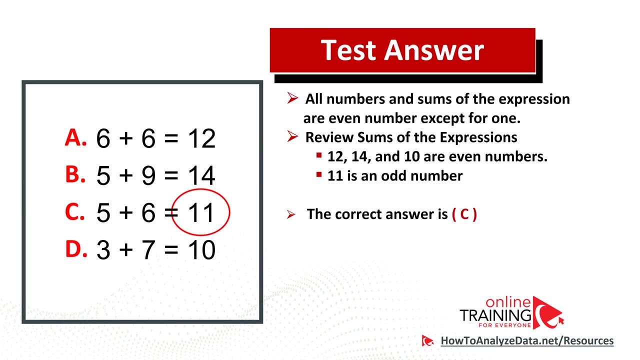 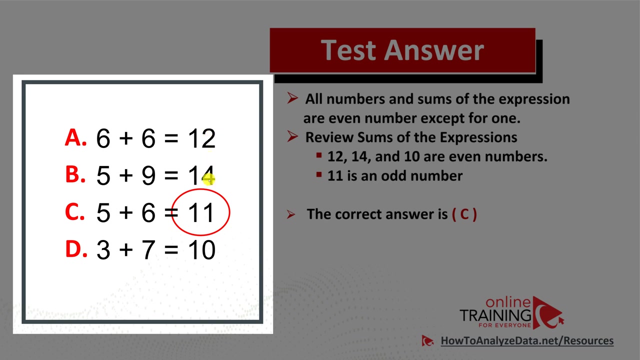 10 or 20 seconds and see if you can come up with the solution. did you come up with the answer? let's continue to see if we can solve this challenge together. let me show you two ways you can solve this challenge. first, let's look on the right side of the expression. you see that the 12, 14 and 10 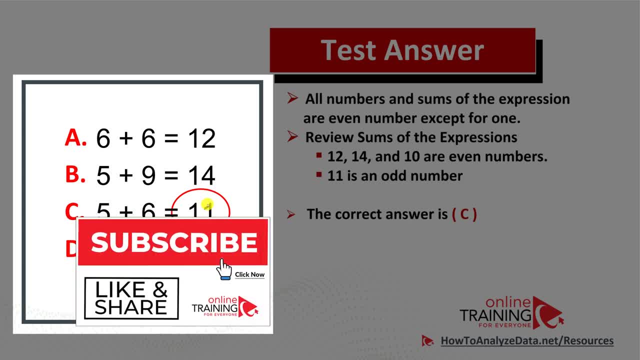 are all even numbers and 11 is the odd number, so that should give you some clues. if you look on the left side of the expression, you see that 6 plus 6 is the combination of four numbers, and the right side of the expression is the combination of: 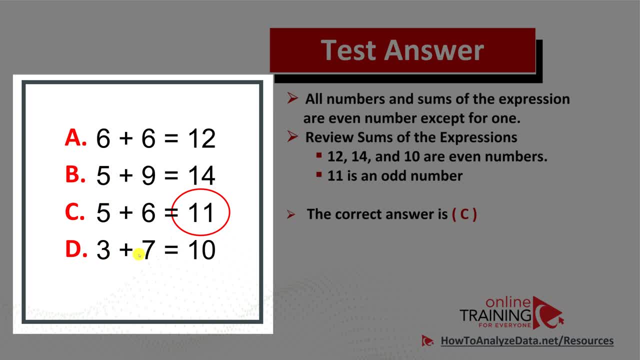 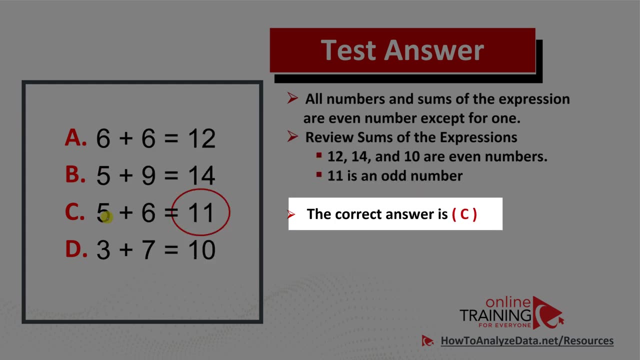 even numbers and you see that 5 plus 9 and 3 plus 7 is the combination of odd numbers. so expression C stands out because you have combination of odd and even numbers in the choice C. so the correct answer, as you might have figured out, is choice C and there are multiple ways how you can look for clues to solve. 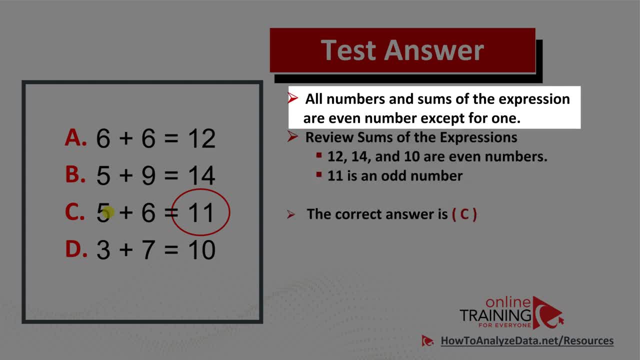 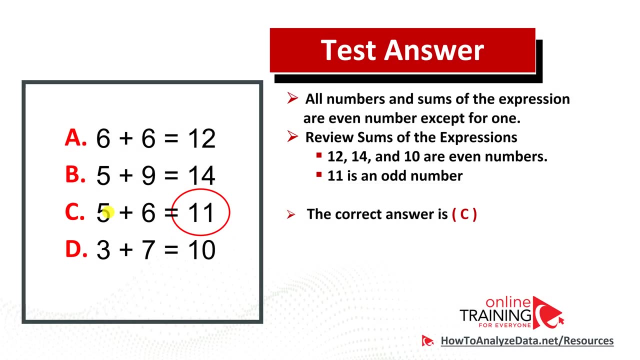 these types of challenges. let's recap: all numbers in the sums of the expression are even numbers except 1. if you review the sums of the expressions, 14 and 10 are all even numbers and 11 stands out. it's an odd number. so the correct answer here is choice c. hopefully you've nailed this question. 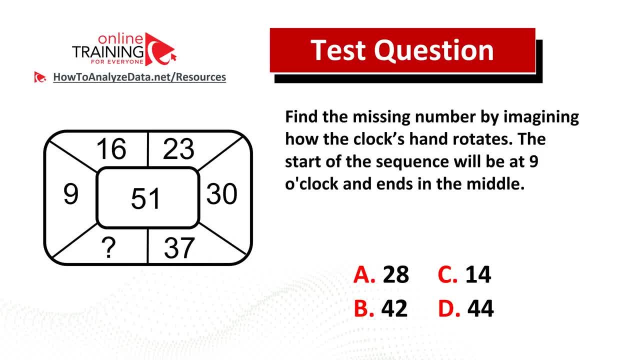 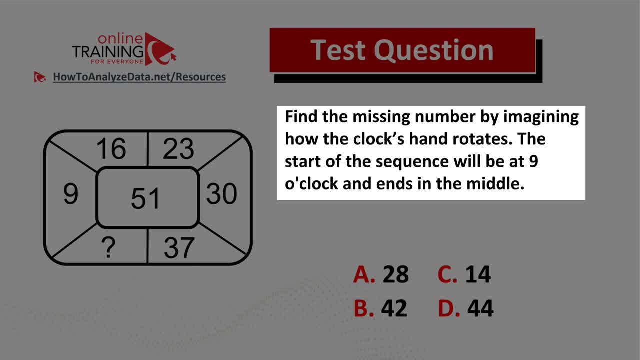 and now here's the question for you to try. please make sure to post your answer in the comment section of this video and i'll give you my feedback. find the missing number by imagining how the clock hand rotates. the start of the sequence will be at nine o'clock and it ends. 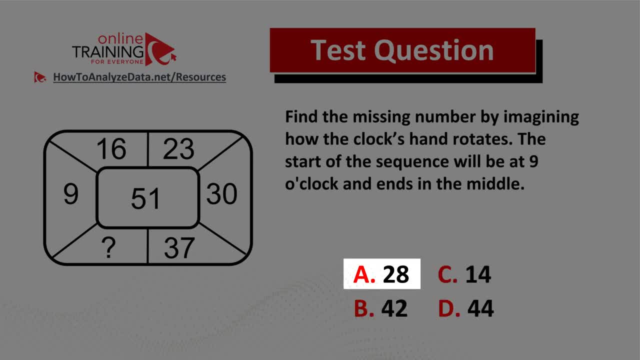 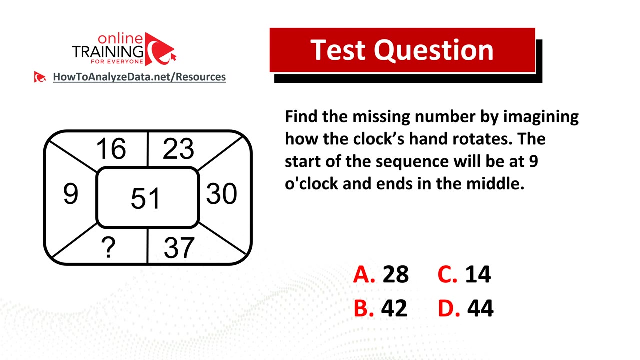 in the middle. you have four different choices: choice a28, choice b42, choice c14 and choice d44. feel free to pause this video and try to solve it and if you came up with the answer, feel free to post it in the comment section of this video and i'll give you my feedback. thanks for participating. 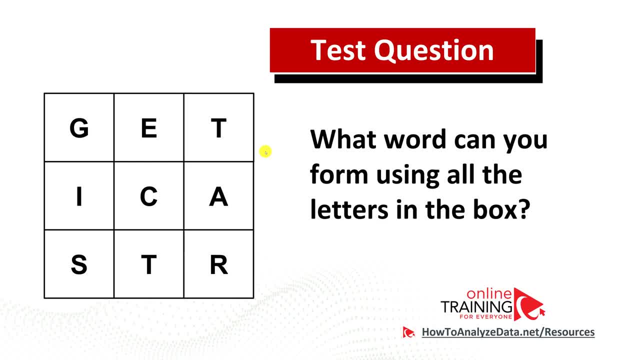 let's look at the very interesting and at the same time tricky question you might frequently see on the test. this particular question tests your imagination as well as the knowledge of the english words. what word can you form using all the letters in the box and you have nine unique letters? 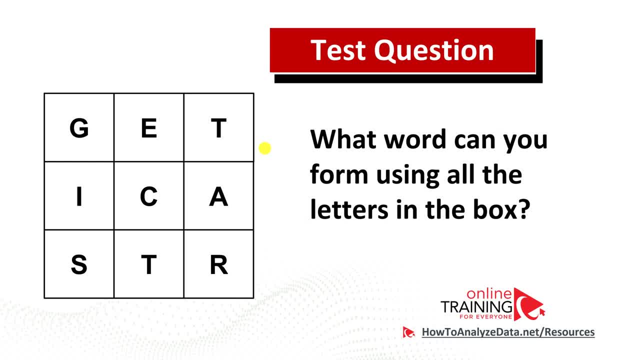 presented in nine different boxes. do you think you know the answer? before we jump to the solution, this might be the right time for you to pause this video to see if you can come up with the solution on your own. do you think you figured out the answer? let's continue. 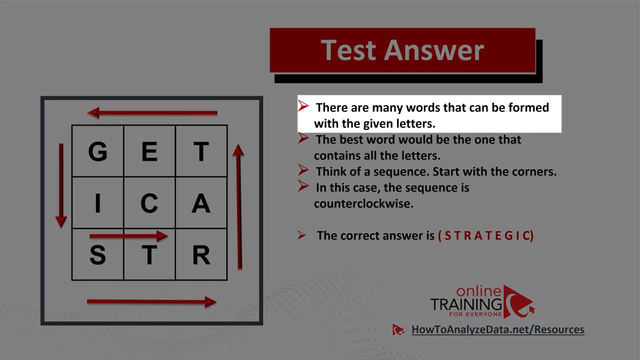 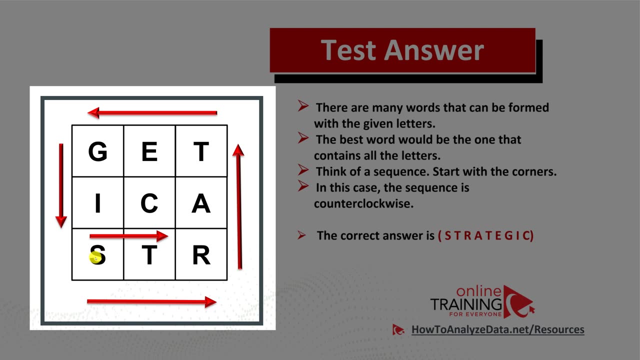 let's see if we can solve this challenge together. obviously, there are a lot of different words that could be formed with the given letters, but what you need to do as part of the test is to find the word that best matches all the letters presented. you should start looking in the corners, and in this case, the pattern is counterclockwise. 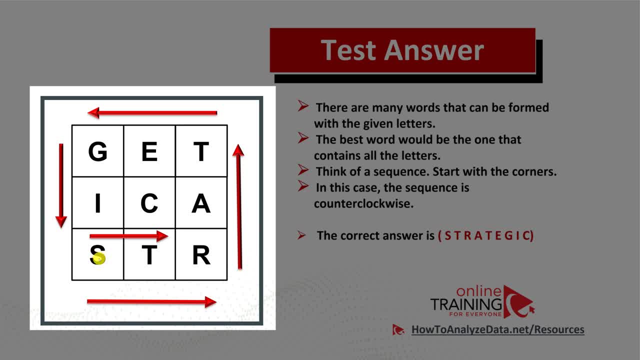 we have the word strategic which is formed starting in the bottom left corner. if you start in the bottom left corner and then flow from right to left, then flow from bottom to the top right and then, and your word in the middle, you will form the word strategic. 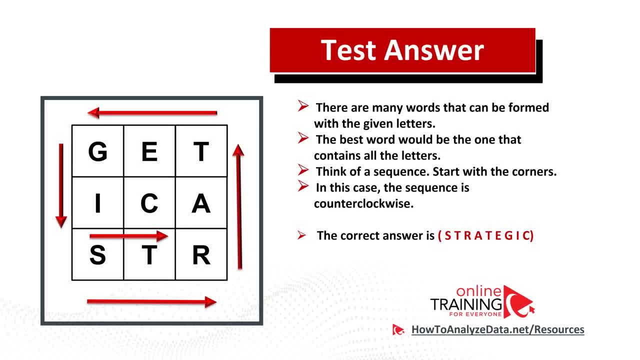 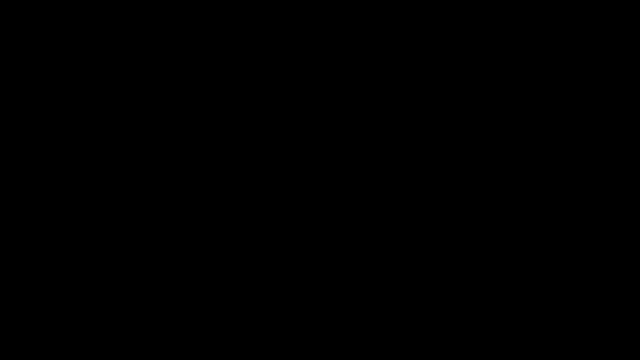 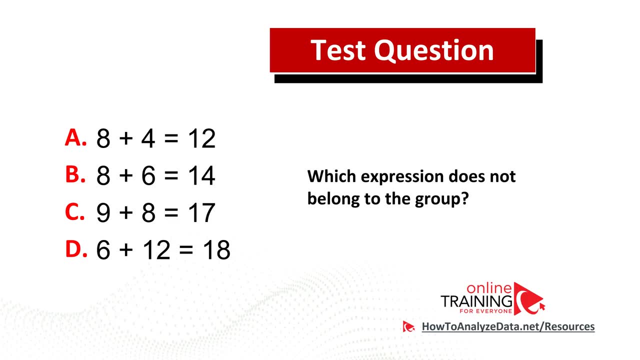 hopefully you've nailed this question, but in case you need more questions or practice problems, please make sure to check out the aptitude test book in the description section of this video. are you ready for this challenging problem? let's look at the very interesting and tricky question you might frequently see on the test which 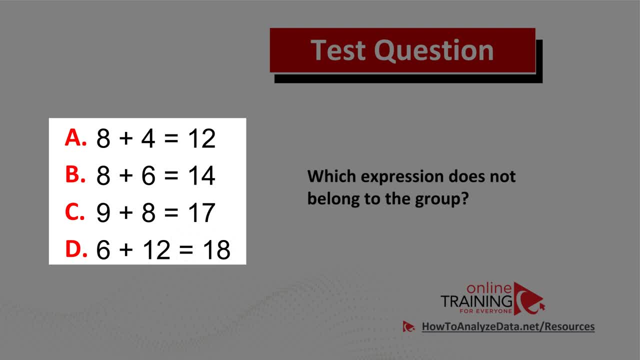 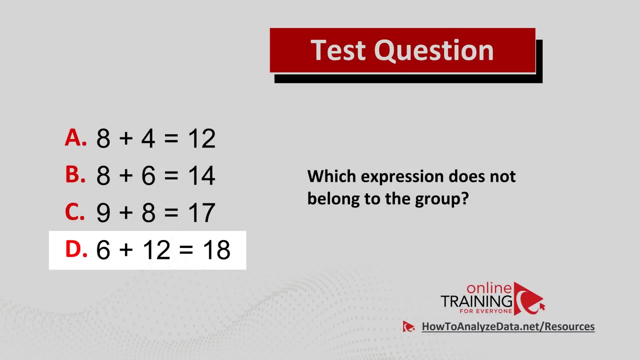 expression does not belong to the group and you have four different expressions: choice a- 8 plus 4 equals 12. choice B- 8 plus 6 equals 14. choice C- 9 plus 8 equals 17. and choice D- 6 plus 12 equals 18. do you think you know the answer now? 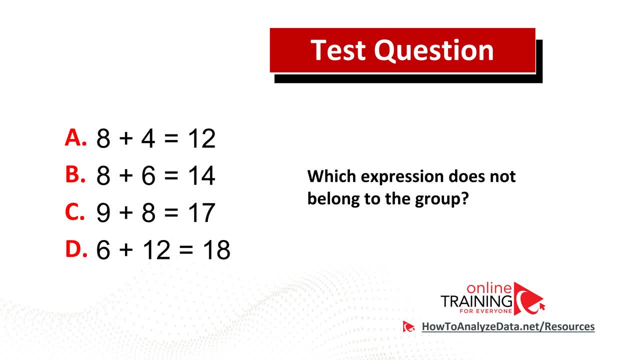 might be the right time for you to pause the video to see if you can come up with the answer on your own. do you think you know the answer? let's continue to see if we can solve this challenge together. what's interesting about this question is the fact that we're dealing here with 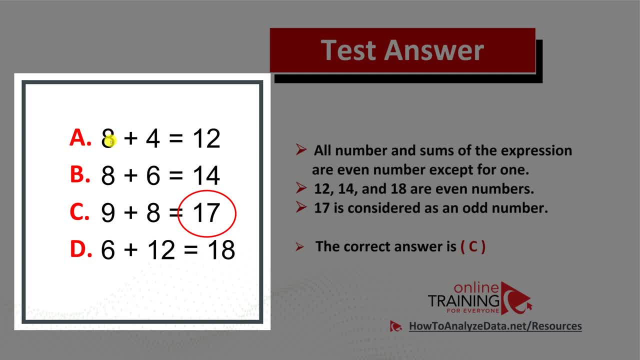 odd versus even numbers. you see that expression a has all the even numbers: 8 and 4 equals 12. expression B is the same thing: 8 plus 6 is 14. all even numbers. same with expression D: 6 plus 12 equals 18. so the expression C has two odd. 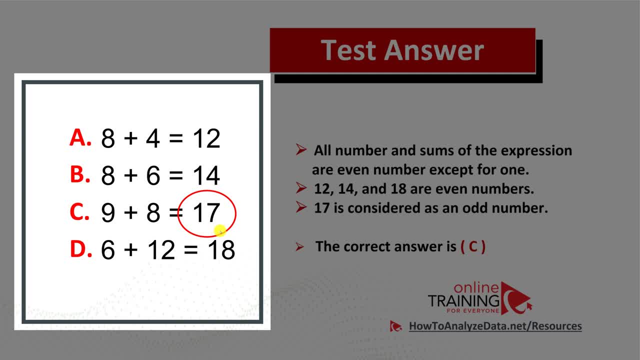 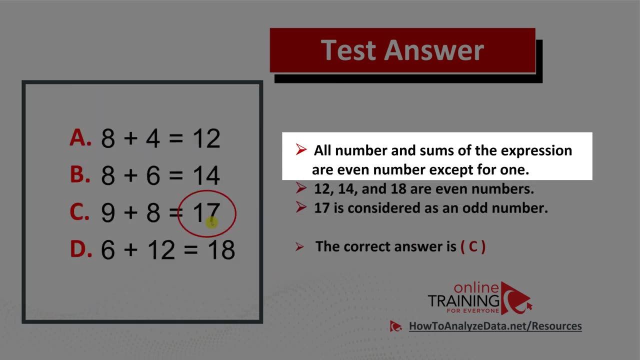 numbers 9 and 17 and if you look at the answers you can also figure it out by just looking at the answer. the answers are 12, 14 and 18 for solutions a, B and D and for the C the answer is 17. so let's recap: all numbers and sums of the expression are even. 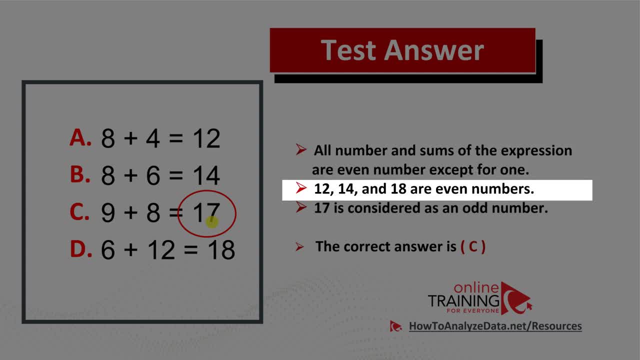 numbers, with the exception of one: 12, 14 and 18 are even numbers, but 17 is the odd number, so the correct answer here is choice C, 17. hopefully you've nailed this question and got to the correct answer on your own, but in case you need more, 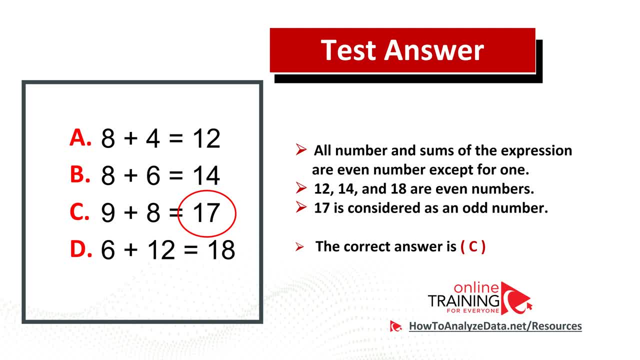 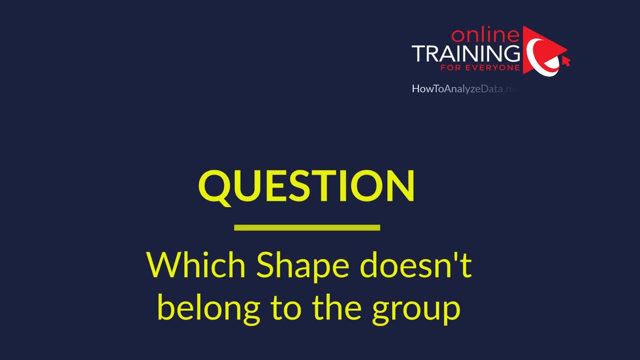 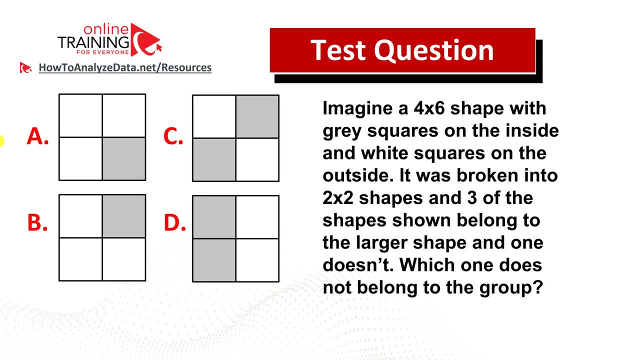 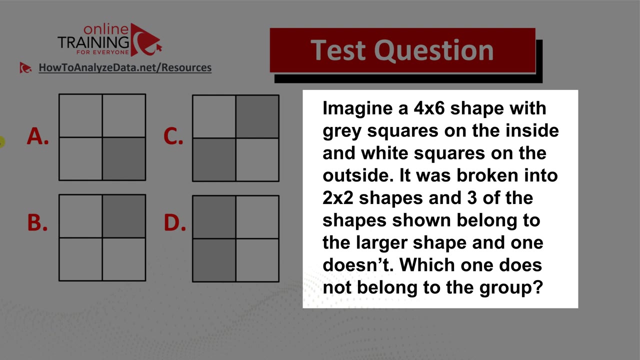 questions or practice problems. please make sure to check out the description of this video for my aptitude test questions PDF ebook. here's the tricky IQ and aptitude test question you might frequently see on the test. imagine a 4x6 shape with gray squares on the inside and white squares on the outside. it was broken into. 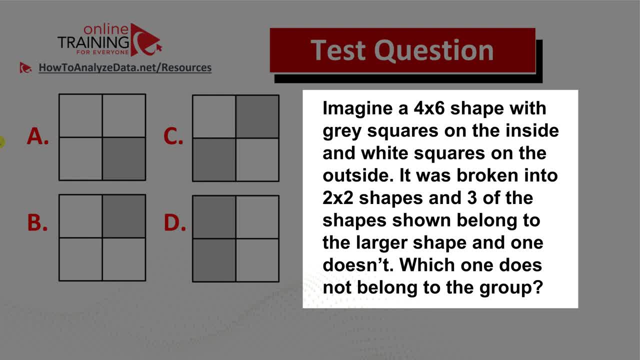 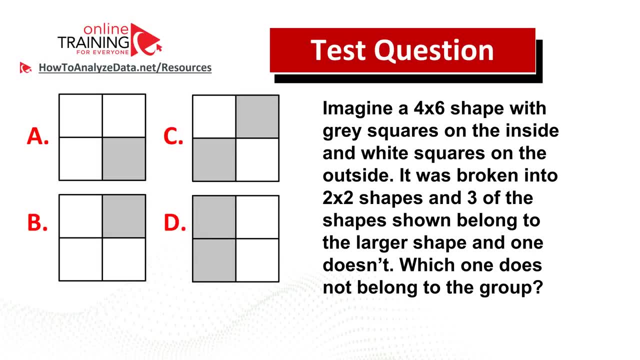 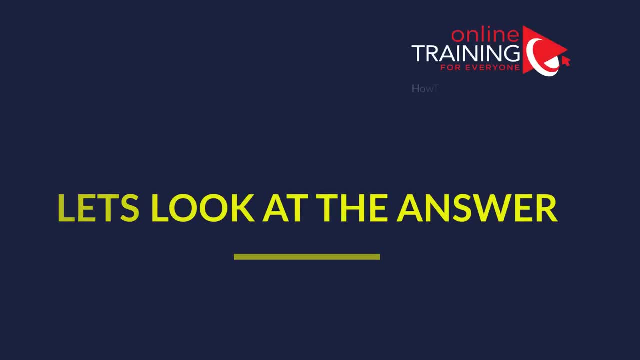 two by two shapes, and three of the shapes shown belong to the larger shape and one doesn't. which one does not belong to the group? do you think you know the answer? now might be the right time to pause this video to see if you can come up with the answer on your own. do you think you came up? 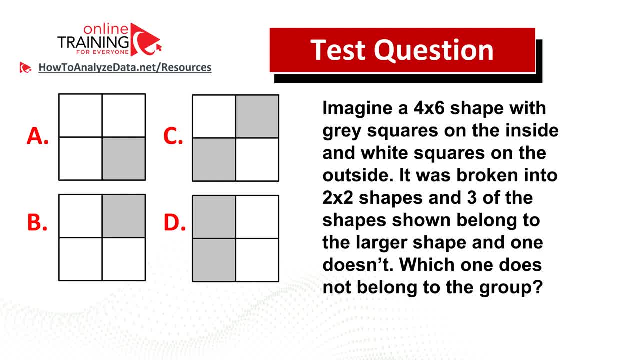 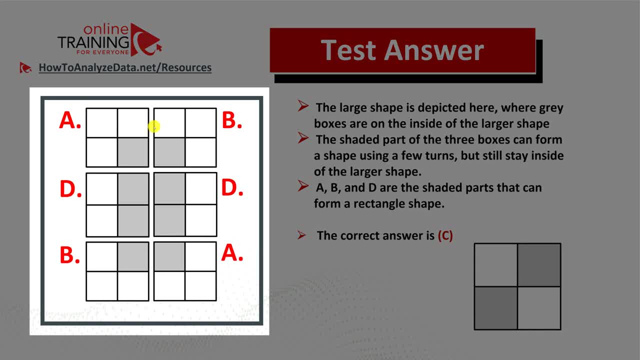 with the answer. let's continue to see if we can solve this challenge together. as you might be well aware, a visual is worth 1 000 words or more. in this case, this is the shape- 4x6 shape- with the gray boxes on the inside and the white boxes on the outside. 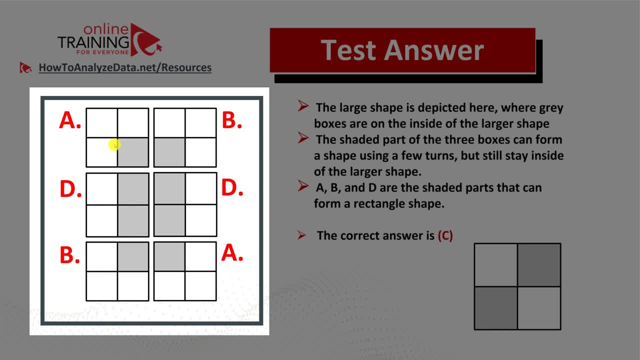 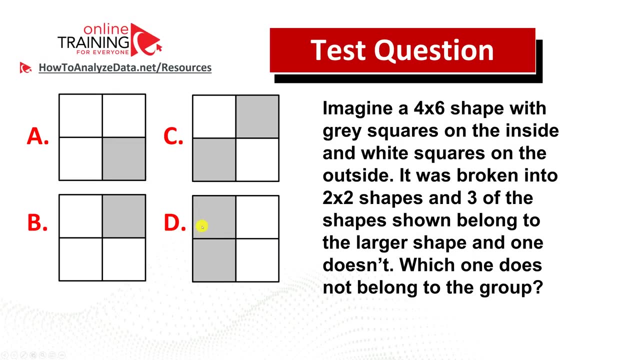 and it was broken down into two by two shapes. if we go back to the question, you see that the choice a is represented right here. if you flip the box in the bottom right corner of the screen, choices B are in the opposite corners and choices D are in the middle. but what you see is that choice. 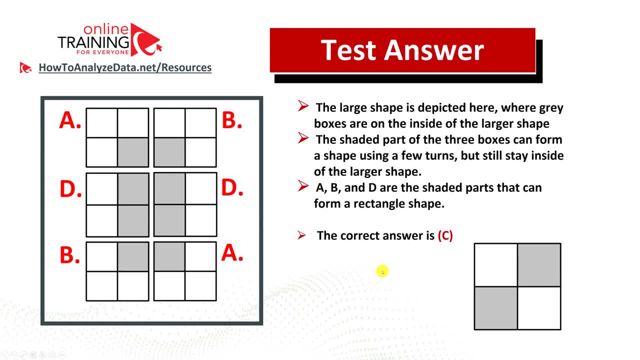 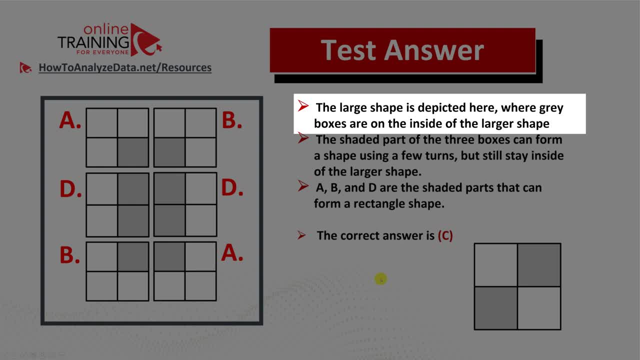 C is not represented here anywhere, so the correct answer here is choice C. let's recap: the large shape is depicted right here where gray boxes are on the inside and the white boxes are on the outside of the larger shape. the shaded part of three boxes can form a shape using few turns, but still say inside the larger shape. this is why choices A, B and D are. 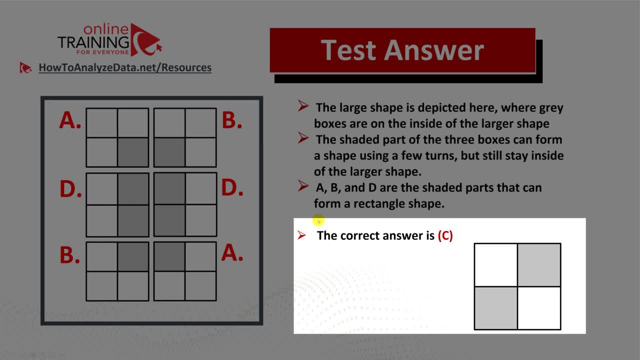 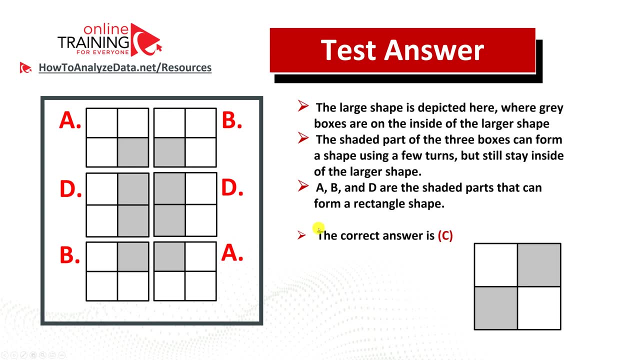 valid choices and choice C is the correct choice and this is the one you should be selecting. hopefully you've nailed this question and answered it correctly, but in case you need more questions or practice problems, please make sure to check out my aptitude test question books. in the description